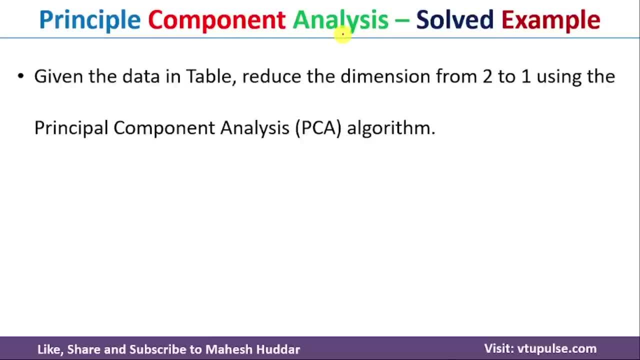 component analysis. To understand principal component analysis, we will take one simple example. In this case, we have been given a data set with the two features and we want to reduce the data set from two dimensional to one dimension. in this case, The data set contains four examples. 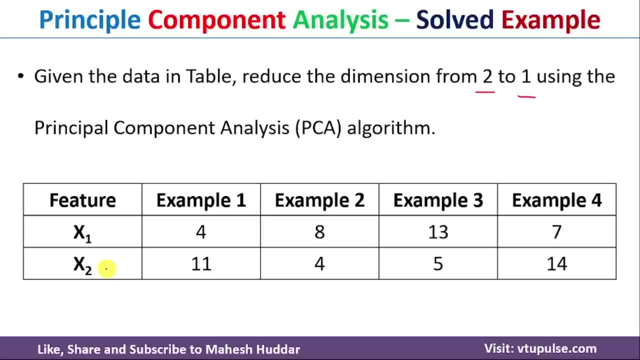 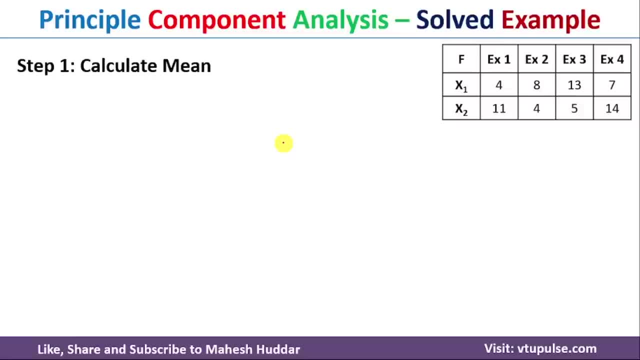 over here, and X1 and X2 are the two features over here. Given this particular data set in principal component analysis, we need to apply multiple number of steps. The first step is to calculate the mean of this particular two features over here. So X1 is the mean of this particular two features over here. So X1 is the mean of this particular two features over here. So X1 is the mean of this particular two features over here. So X2 is the first feature and X2 is the second feature. 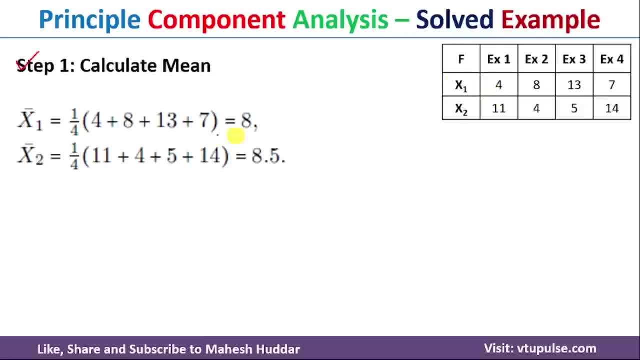 So first we need to calculate the mean of X1 and then mean of X2 over here. So the mean of X1 is represented as X1 bar, which is equivalent to the addition of all these particular four values divided by 4. that is nothing but 8 in this particular case. Similarly, the mean of X2 is: 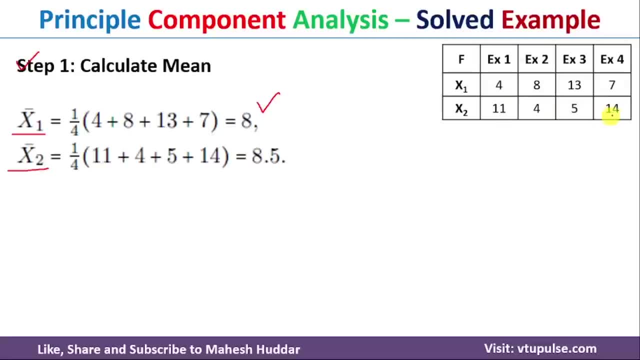 equivalent to X2 bar. again, addition of all these particular feature values divided by 4, which is equivalent to 8.5 in this case. Now, once you calculate the mean, now we need to calculate something called as coherence matrix. The coherence matrix looks. 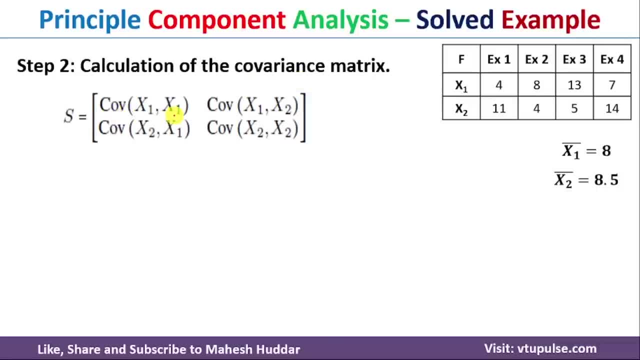 something like this: S is equivalent to covariance of X1- X1, covariance of X1- X2, covariance of X2- X1, covariance of X2- X2 over here. Now the next question comes in front of us is how to calculate the covariance of X1- X1 over here To calculate covariance of X1- X1,. 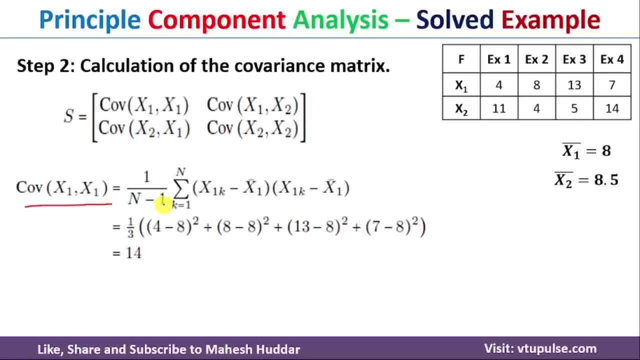 we use this particular formula, which is equivalent to 1 divided by n minus 1.. n is the number of examples given to us. So in this case we have been given four examples. So the value of n is equivalent to 4 here. Summation of k is equivalent to 1 to n here. 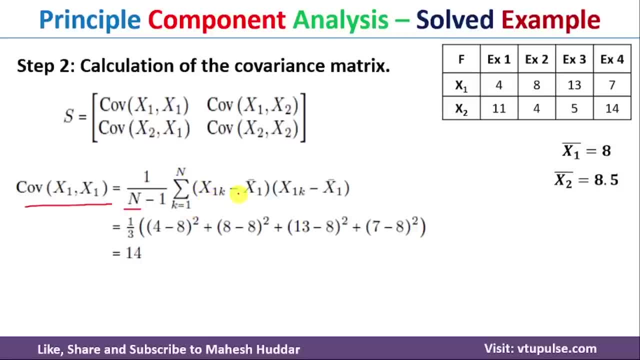 and then X1k minus X1 bar. X1k is nothing but X11, X12, X13, X14. over here, that is 48137. in this case, multiplied by the second one is again X1.. So X1k minus X1 bar, over here, X1 bar we have. 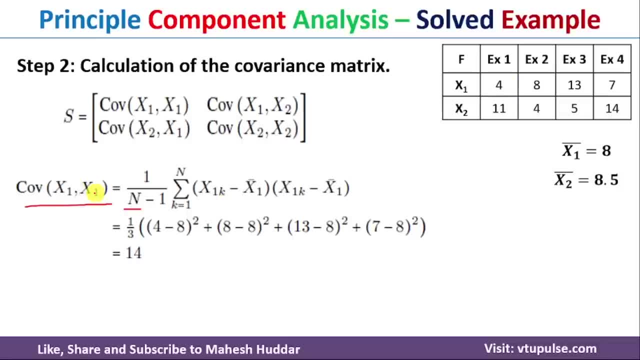 already calculated and because both the cases we have X1, X1 here, So it will become X1k, here also X1k. So that is the reason: it will be nothing but the square of this particular bracket here. Now we will put the values: X1k is 4.. Again, this X1k is also 4.. Second time it will become 8,. 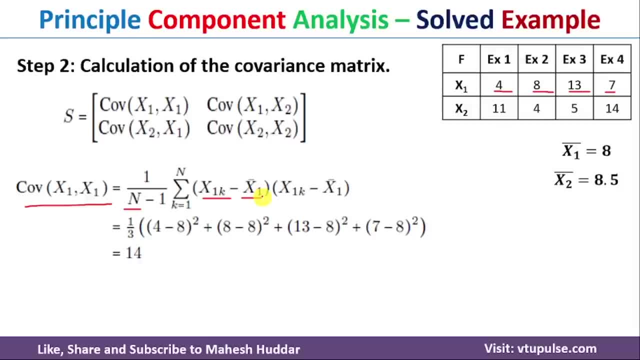 third time it will be 13 and fourth time it will be 7 over here. X1 bar is nothing but 8 in this particular case. So every time it will be 8- 8 over here, and once you solve this particular equation, you will get 14 as the covariance of X1- X1 over here. Now, coming back to the covariance, 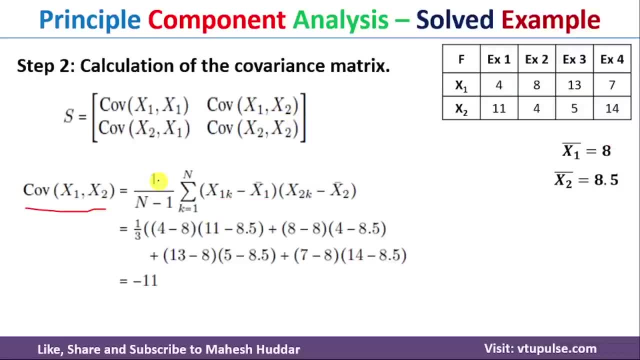 of X1- X2.. So covariance of X1- X2 is equivalent to 1 divided by n minus 1. again k is equivalent to 1 to n, that is, n is equivalent to 4 here. X1k minus X1 bar. Now it is X2k minus X2 bar here. 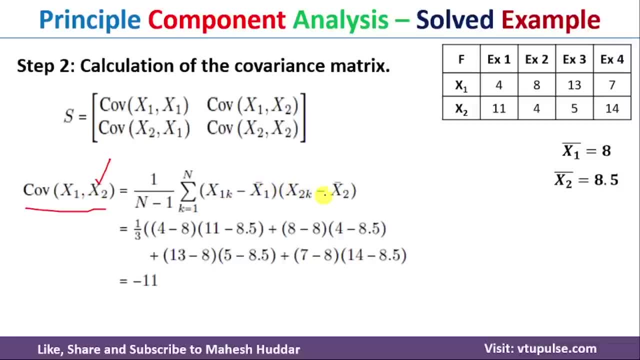 because the second one is X2 over here. So that is the reason it is X2k minus X2 bar. over here Again, X1k is nothing but X1 bar over here, So that is the reason it is X2k minus X2 bar over here. 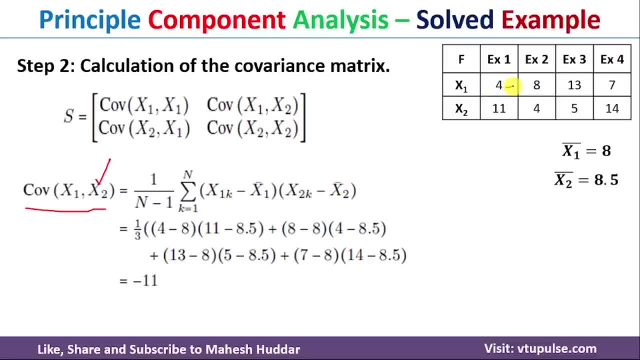 Again, X1k is nothing but X1k minus X2 bar over here. So that is the reason it is X2k minus X2 bar over here. In the first case it is X11, X12, X13, X14. that is nothing but 4,, 8,, 13 and 7 minus this value. 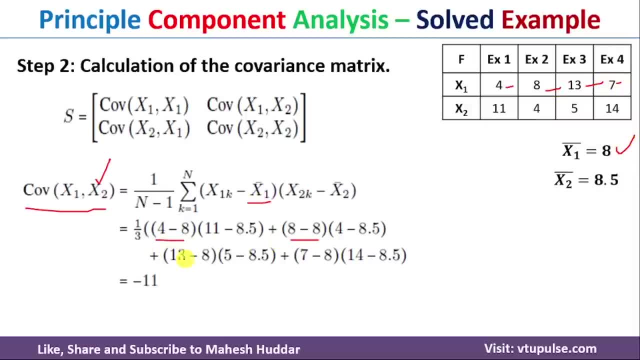 that is 8 over here, So that is what I have written. This is the first time, second time, third time and fourth time over here. The second one, that is X2k. X2k is nothing but X21,, 22,, 23,. 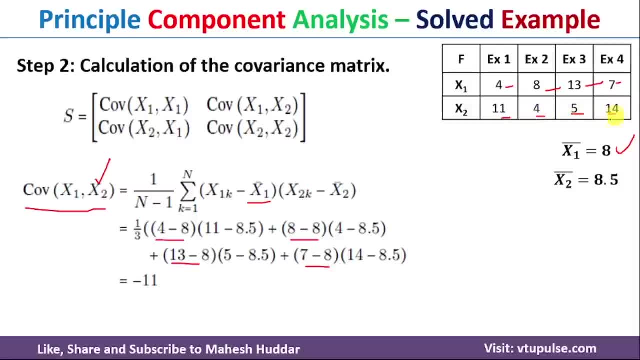 24, that is nothing but 11, 4, 5 and 14 minus 8.5 in all the cases. So 11 minus 8.5,, 4 minus 8.5,, 5 minus 8.5 and 14 minus 8.5.. So that is the reason. it is X2k minus X2k. So that is the reason. 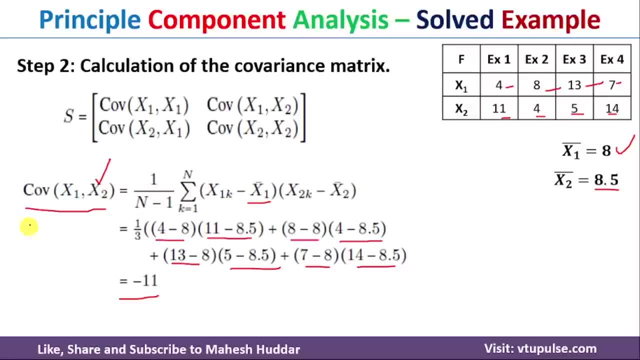 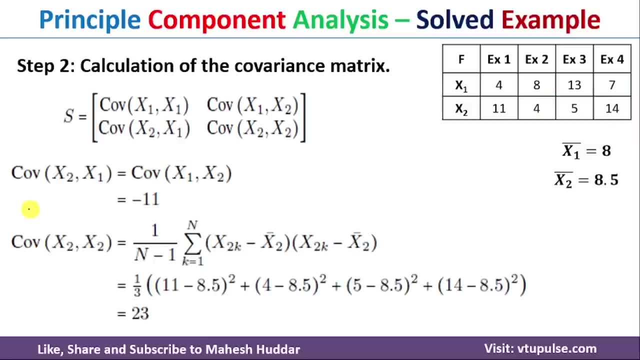 once you solve it, you will get minus 11 in this case. so once you calculate the covariance of x1- x2, that is nothing but the covariance of x2- x1 also that will come and sit over here. so that's reason i have written: covariance of x2- x1 is also minus 11 in this case. similarly, we need to. 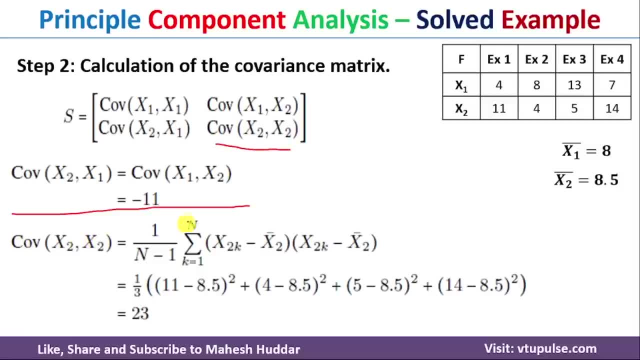 calculate the covariance of x2- x2. covariance of x2- x2 is equal to 1 divided by n minus 1. summation of k is equal to 1 to n. here again, this will be x2k minus x2 bar. x2k minus x2 bar here. 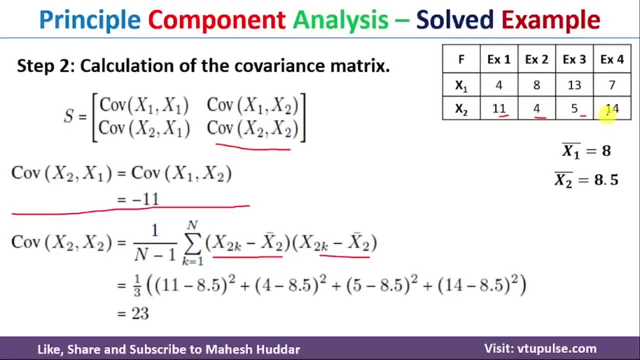 2k is nothing, but what? 2, 1, 2, 2, 2, 3, 2, 4 and x2 bar is 8.5 in all the cases. so once you solve this equation again, you will get 23 as the covariance over here. now we need to put all these particular. 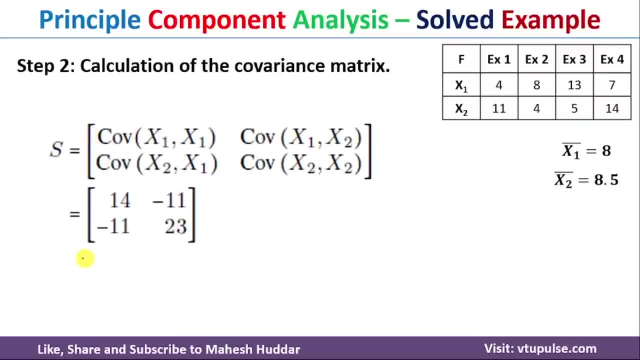 four values to get this particular covariance matrix. so the covariance matrix looks something like this: 14 minus 11 minus 11, 14 minus 11 minus 11, 14 minus 11 minus 11 minus 11: 23 over here. so this is the second step. we need to calculate the covariance matrix. 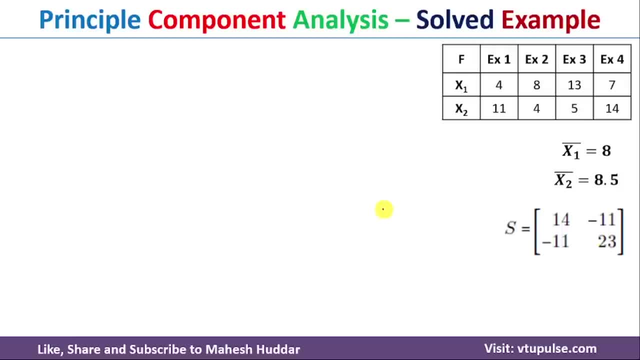 this is how the covariance matrix looks like. now, in the third step, we need to calculate the eigenvalues of this particular covariance matrix. to calculate the eigenvalues of this covariance matrix, use this equation: that is: 0 is equivalent to determinant of covariance matrix minus lambda i. i is the identity matrix in this case, so s is already known to us- minus lambda i. 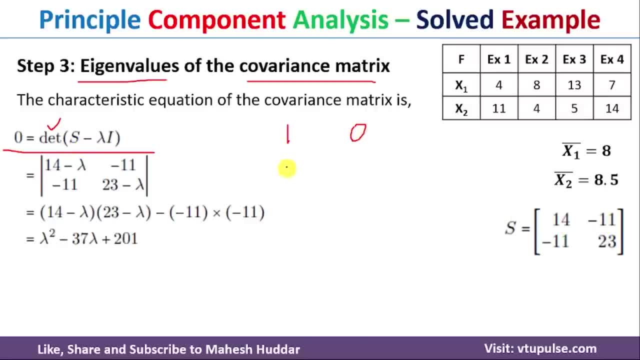 i is the identity matrix. that's the reason it will be something like this: one 1 0, 0, 1 over here. so if you multiply by lambda, it will become lambda 0, 0 lambda over here. now, if you subtract it from s, it will. 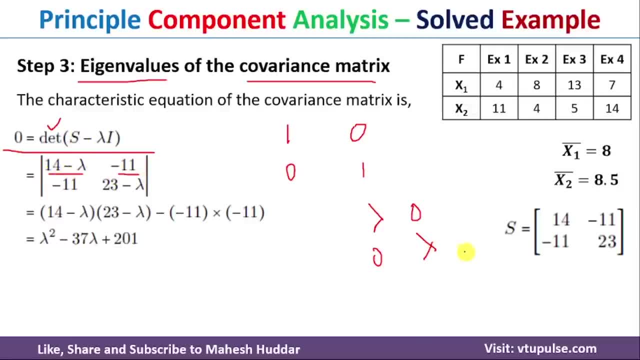 look something like this: 14 minus lambda, this will be 11 minus 0 over here. so it will become minus 11 only. and the second time it will be again here minus 0 over here it will be minus 11 only. 23 minus lambda. because we have to calculate the covariance matrix, so we need to calculate the. 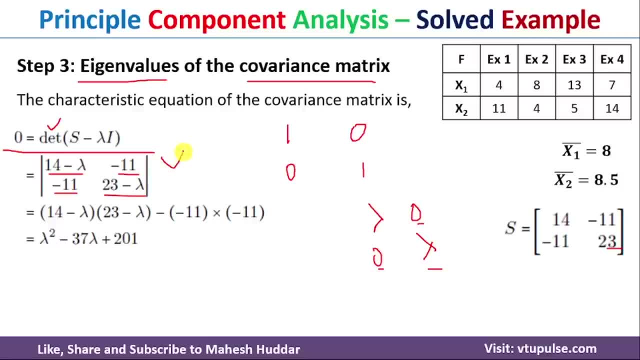 covariance matrix. we have 23 here minus lambda over here. so it looks something like this and we know how to calculate the determinant of any matrix. the determinant is in this case 14 minus lambda multiplied by 23 minus lambda, this one minus minus 11 into minus 11. so this particular 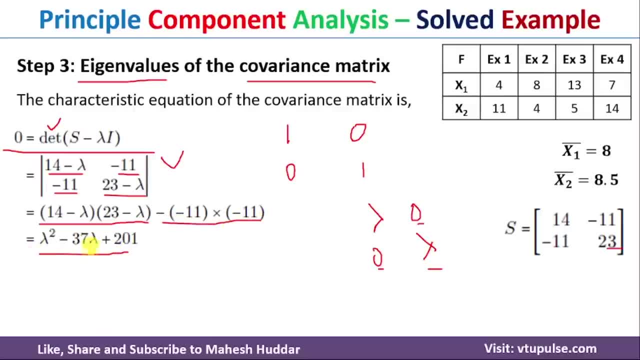 term. and if you solve this particular equation you will get lambda square minus 37, lambda plus 201, which is equivalent to 0 here now it's a quadratic equation. you can use your calculator to come up with the lambda values over here. that's the covariance matrix. so if you solve this, 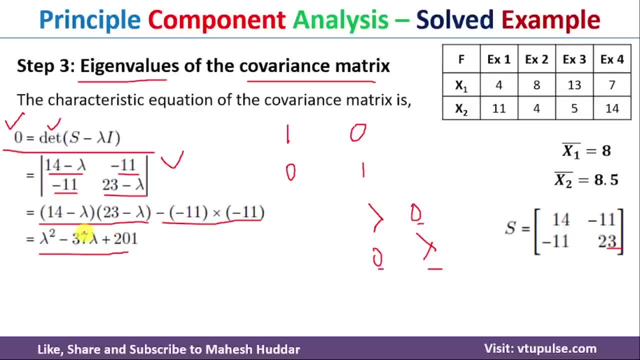 is nothing but the roots of this particular quadratic equation. once you calculate the roots of this particular quadratic equation, you will get the first root as 30.3849. second one is 6.6151. so you can say that this one is the lambda 1 and second one is lambda 2. over here now in the fourth. 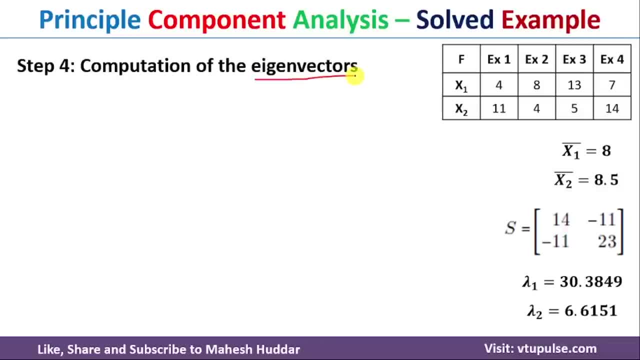 step we need to calculate something called as eigenvectors over here. to calculate eigenvector, we will name the eigenvector as u is equivalent to u1, u2. we use this particular equation, that is s minus lambda i. s is a coherence matrix. i is the identity matrix, u is the eigenvector over here. 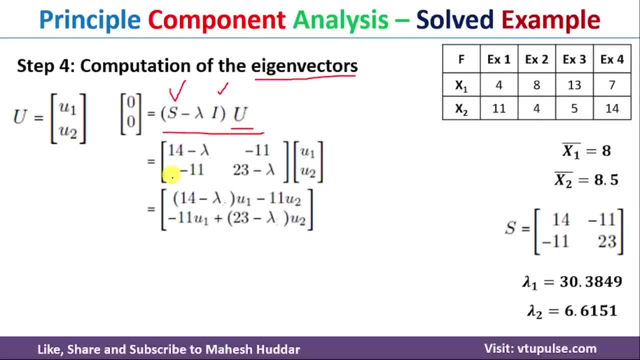 which is equivalent to 0. so we know all this particular thing. if you put all those particular thing, it will look something like this, and then this will be: this row is multiplied to this particular column. it looks like 14 minus lambda into u1, minus 11 into u2. so that is the first. 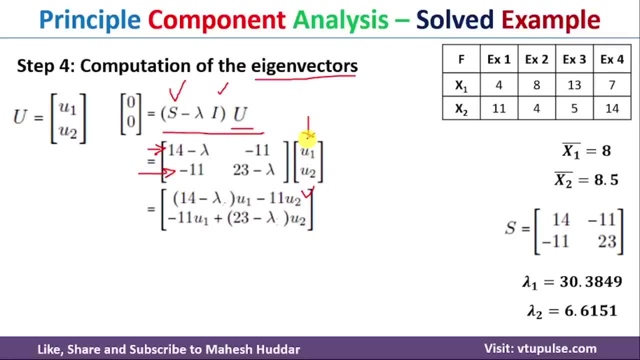 line. here again, this row is multiplied to this particular column, so minus 11 into u1, plus 23, minus lambda into u2 over here. so you will get these two equations, which is equivalent to 0, 0 in this particular case. now what we need to do is we need to solve this particular equation so that you will. 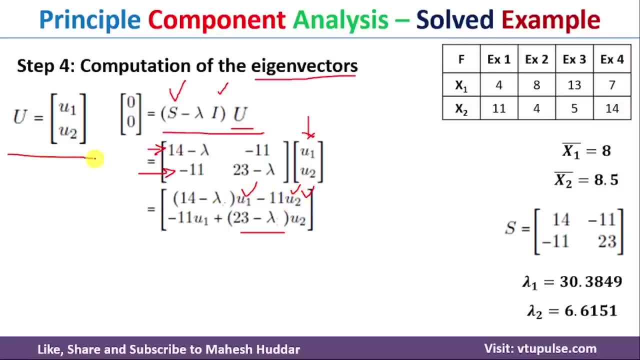 get u1 and u2 value here. once you get the u1 and u2 value, that is nothing but your eigenvector over here. now we will take either the first equation or second equation to get the value of u1 and u2 in this particular case. i have considered the first equation here. 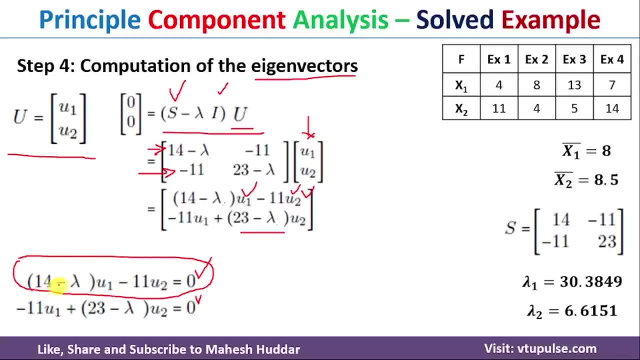 so now, if you look at this particular equation, it is nothing but 14 minus lambda, u1 is equivalent to 11 u2. that is because, if you take this side, no, it will become plus. over here now you can say something like this: 14 minus lambda multiplied by u1 is equivalent to 11 u2. over here. now what? 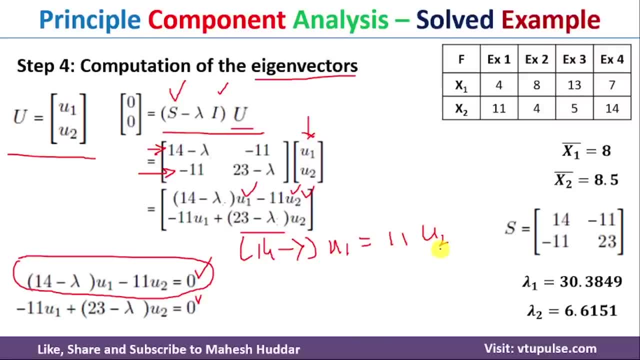 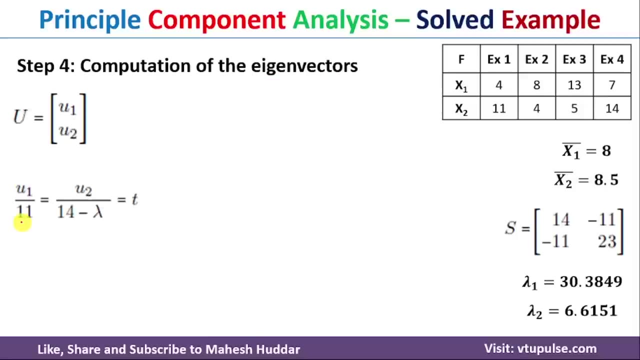 i will do. i will take 11 this side and 14 minus lambda this side over here, so it will become u1 minus u1 divided by 11, which is equivalent to u2 divided by 14 minus lambda over here. so we will set it to t here for both the values. so it will look something like this: u1 divided by 11, which. 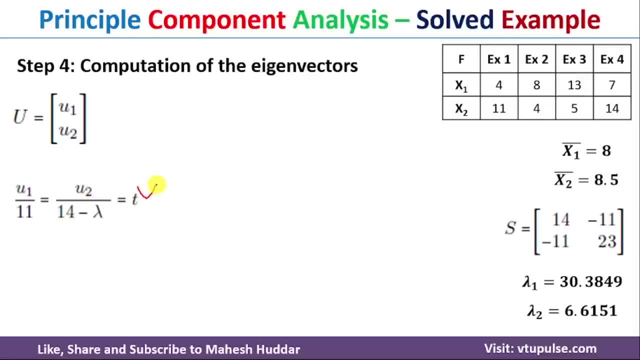 is equivalent to u2 divided by 14 minus lambda, which is equivalent to t. here again, if you solve this particular thing, uh, u1 is equivalent to 11 t and u2 is equivalent to 14 minus lambda multiplied by t. over here, we assume that the value of t is equivalent to. 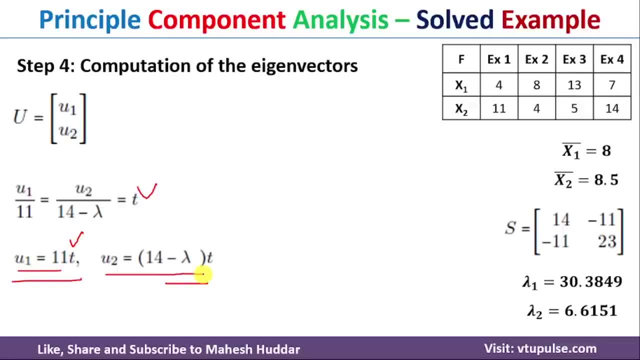 so u1 will become 11 and u2 will become 14 minus lambda over here. so your u1 will become or. you can say that this u will become, you can say that 11, and the second one is 11 minus lambda over here. this is the eigenvector for the given. what is that called as a coherence matrix here? 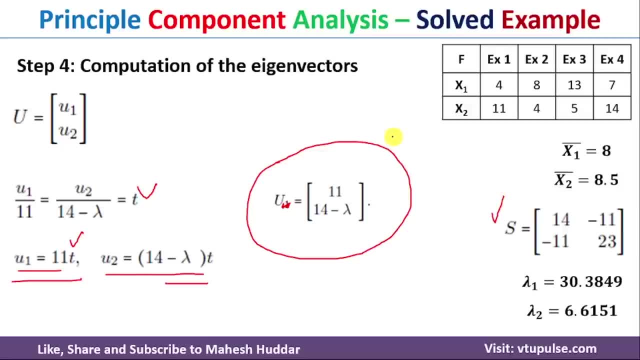 now the next thing is: whenever we want to calculate the principal components, we have to consider the largest eigenvalue. here we have two eigenvalues, lambda 1 and lambda 2. between these two, this is the largest one. so we need to consider this, and then we need 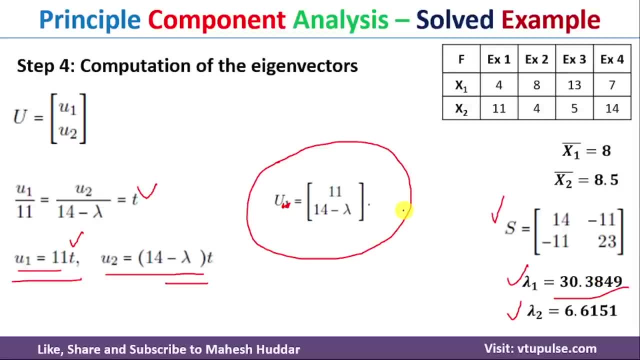 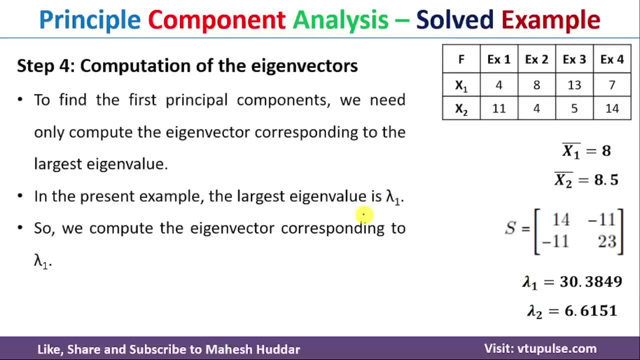 to calculate the principal components over here. if you want one more principal component, we need to consider the next eigenvalue and so on. so in this case we want only one principal component. so that's the reason i will consider lambda 1 over here. u will become 11, 14 minus lambda 1 in. 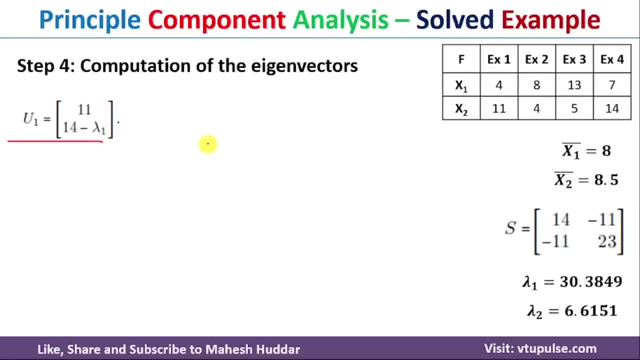 this particular case. so this is how actually the eigenvector will look like over here. now what we need to do over here is we are not much interested in this eigenvector. we are interested in unit eigenvector. so that is the reason. what we do here is we will first calculate the length of this particular u1. 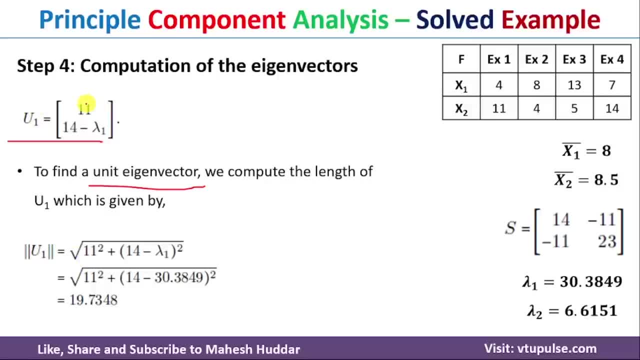 the length of u1 is equivalent to square root of 11 square plus 14, minus lambda 1 bracket square over here, which is equivalent to 19.7348. because lambda 1 is known to us, you need to put it over here and then you need to solve here. so the length of unit eigenvector is equivalent to: 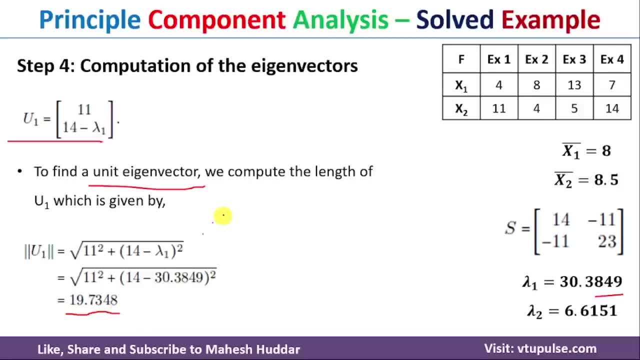 19.7348 over here. so the final eigenvalue or the eigenvector will look something like this: for the first one, for lambda 1, you can say e1 is equivalent to this: 11 divided by for the length of u1 divide, and the second one is 14 minus lambda 1 divided by this particular, the length of that. 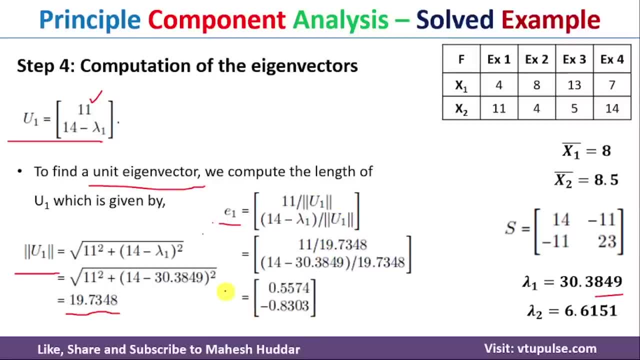 unit eigenvector over here. so put all those particular values: e1 will become 0.5574 as the first value, minus 0.8348 over here. so this is the length of unit eigenvector over here. so this is 0.8303 as the second value over here. similarly, if you want one more eigenvector, you need to put: 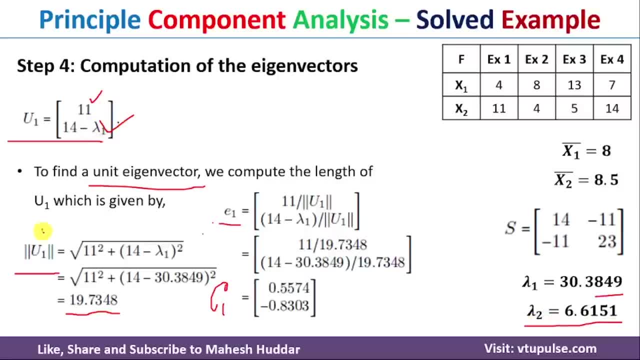 this particular lambda 2 over here. that's the first thing, and then you need to calculate the unit length, and then you need to calculate e2 here. so e2 in this particular case is 0.8303 and second one is 0.5574 over here. so this is e1 and this is e2. we are not much interested in. 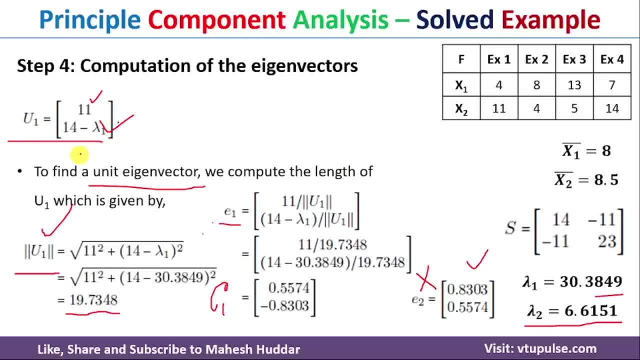 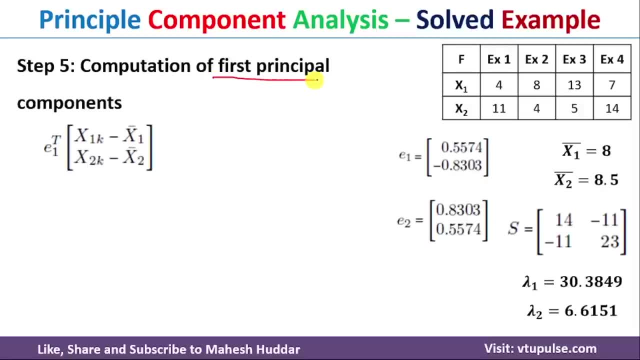 e2. so that's the reason i have not shown the calculation here, but it's very easy. so we have calculated the eigenvector, that is, e1 as well as e2 in this particular case. so we have calculated this particular case. now what we need to do is we need to calculate the principal components that. 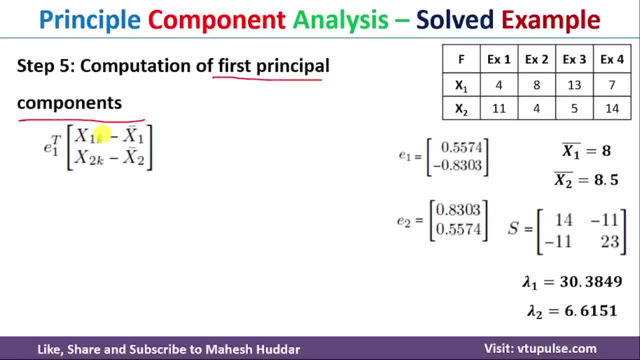 is the fifth step over here, how to calculate principal components. this is the equation we need to use. we have already calculated the eigenvector. we need to take the transpose of that one multiplied by x1k minus x1 bar, x2k minus x2 bar over here. so in the first case, x11, x21, x11. 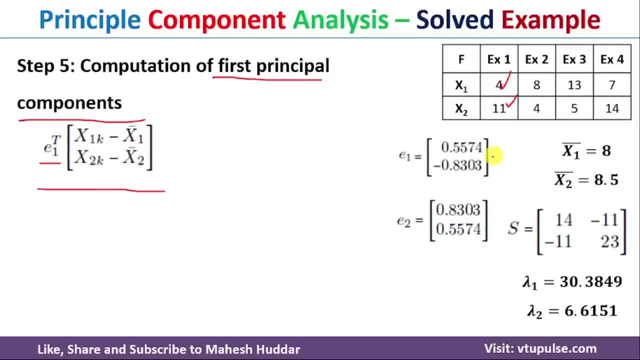 so that value i need to put. so, for example one, we will get the principal component. in the second case, i need to put 8 for x12 and 4 for x22 over here, and then we will get the principal component. for second example, and the same thing will be repeated for two more examples over here, i will 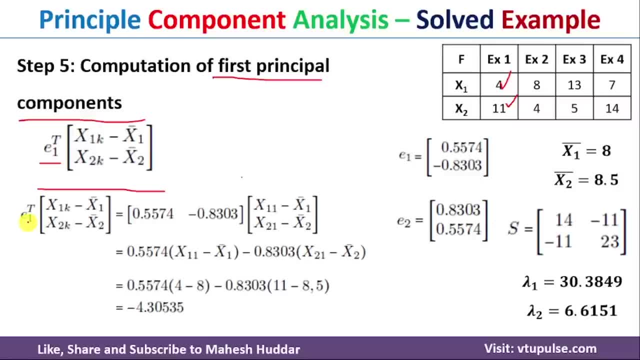 show one calculation here. in this particular case, e1 transpose x1k minus x1 bar, x2k minus x2 bar is equivalent to this. one is already known to us. i have written the transpose of that particular e1 here: and x- the first case k- will be 1 over here, x11. 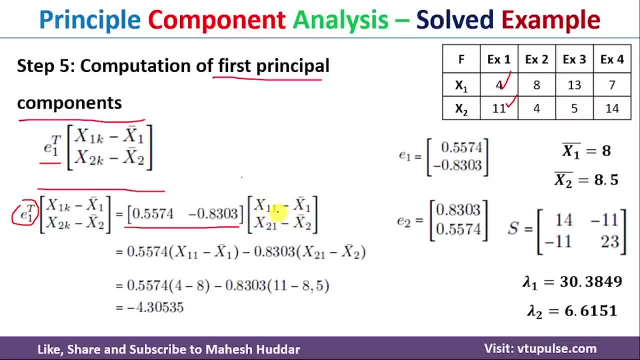 minus x1 bar, x21 minus x2 bar over here. so this is known to us, that is 4. this is known to us, that is 11. x1 bar is known to us, that is 8. x2 bar is known to us, that is 8.5. we put all those particular. 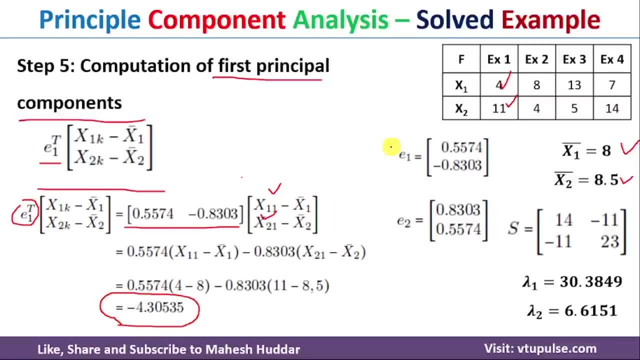 values you will get. the first principal component is: with respect to the example one is minus 4.30535 over here. now the same thing has to be repeated for example 2. in example 2, only change will take space over here. this x11 will replace with x12 and x21 will be replaced with x21. that is nothing, but this will. 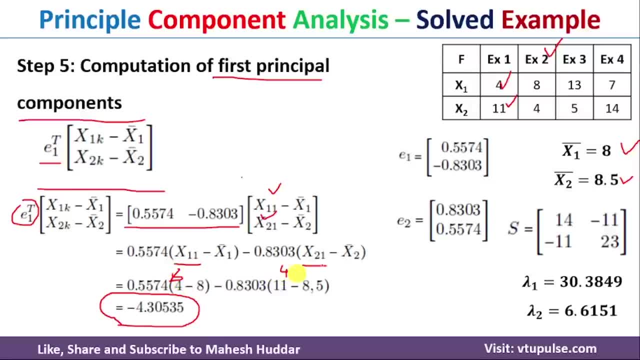 be 8 over here and this will be 4 in this particular case. similarly, in the second next case, this will become 13 and this will become 5. in the last case, this will become 7 and this will become 14 in that particular case. so once you calculate the principal components for all the examples, 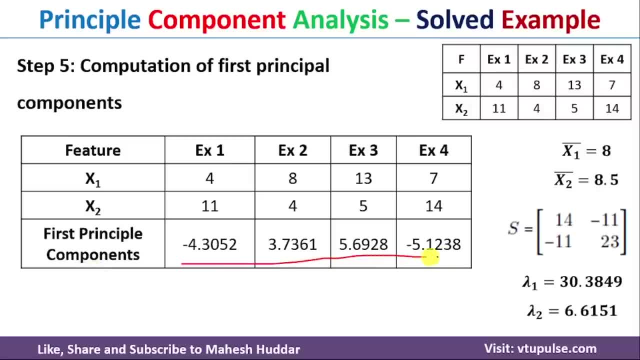 the principal components for the first eigenvector looks something like this: these are the four principal components with respect to four examples over here. now, what we did here is we have been given two features, x1 and x2. we have reduced this particular features into one feature, that is first. 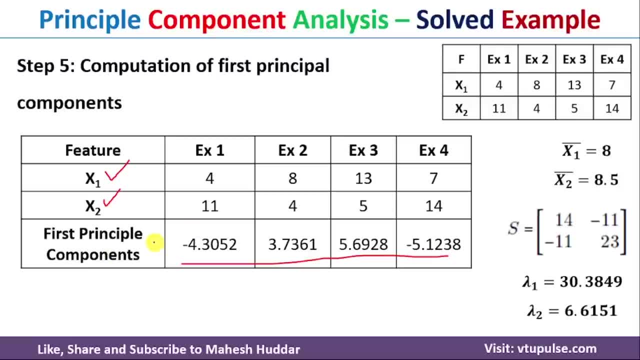 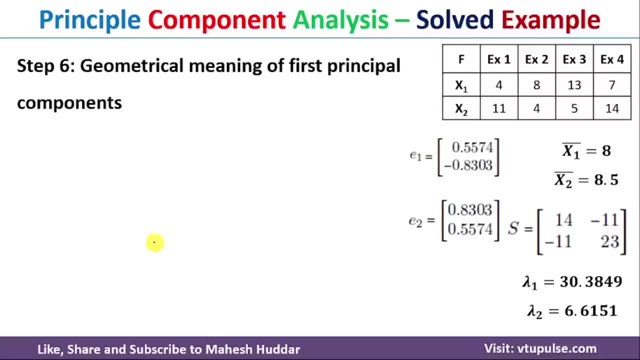 principal component here. similarly, if you want one more feature, you can calculate the second principal component, and so on. now we will try to understand the geometrical meaning of this principal components. so this is how, actually, we have already calculated the principal components, we have already drawn this particular two features. so these particular dots will indicate the data. 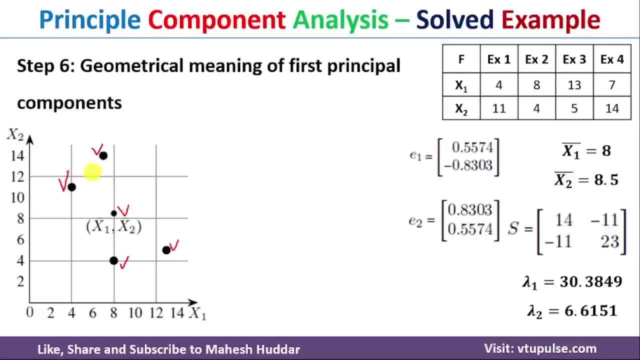 points and this will indicate something called as the mean of this particular data set over here. now what i need to do over here is i need to draw this particular eigenvectors over here, so that can be done something like this. so first i need to draw a horizontal line from this particular mean. 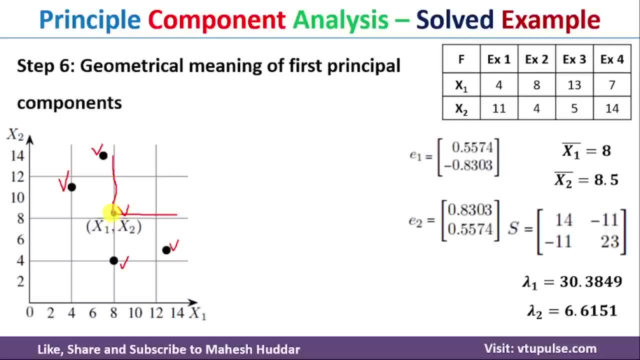 and then vertical line from this particular mean here and this one we will assume it as zero. zero now, and the first eigenvector value is point five, five, seven, four. so this is a positive value minus 0.8303. so somewhere here we will get that. 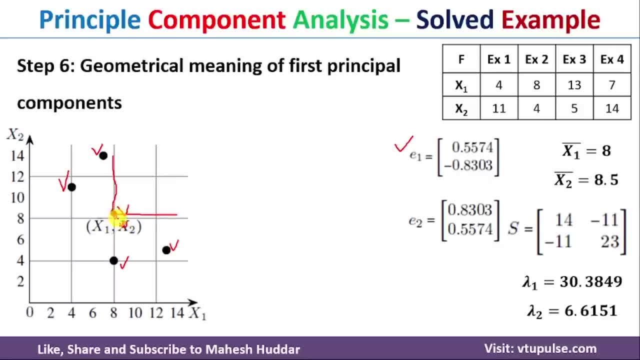 particular thing. so what we need to do here is from this particular origin toward this one. we need to draw one line here, so this will become your e1. similarly e2. e2 contains what? 0.8303. so this is zero, zero, 0.8303. right side, the y value is 0.5574. so upward direction somewhere here you.